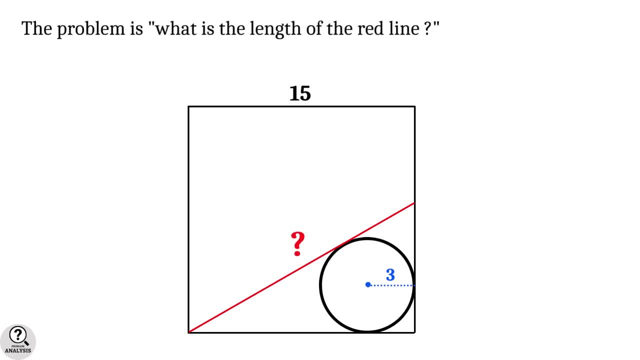 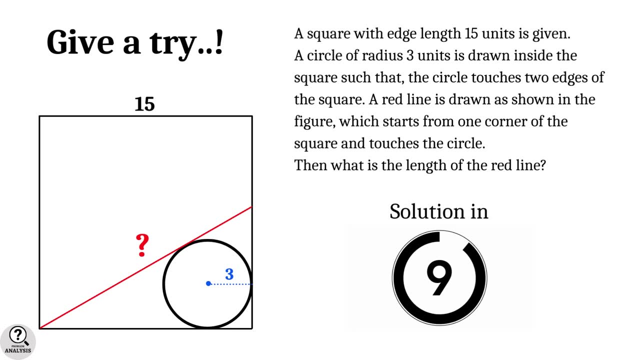 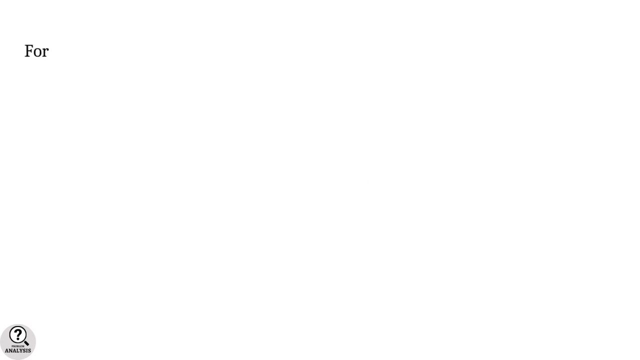 my problem is: what is the length of this red line? If you want to attempt the problem, pause the video and just give a try, And the solution is right here. First, let's give some notations to each vertex. The square is denoted by ABCD. the red line is denoted by DE. center of the circle is named as O. 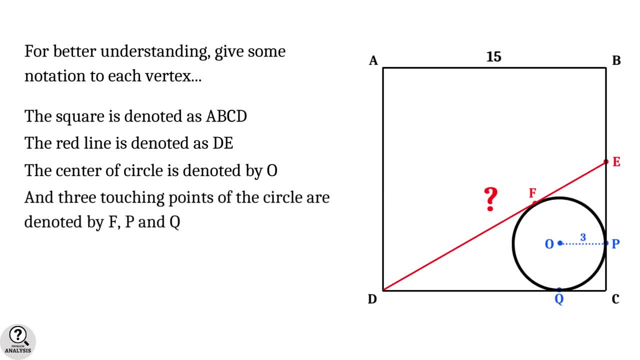 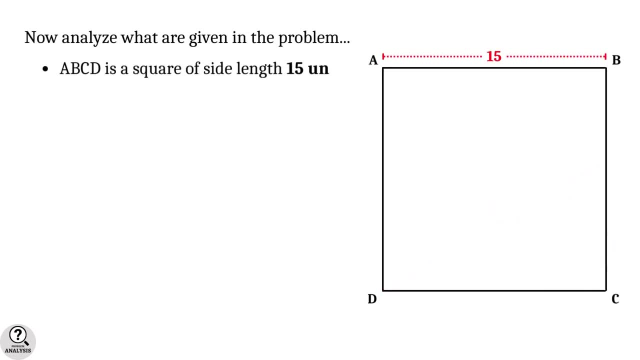 and finally, the three touching points are denoted by F, P and Q. Now we are going to analyze the problem. Firstly, ABCD is a square of 15 units side length. Secondly, radius of the circle is 3 units. And then the lines BC, CD and DE are touching. 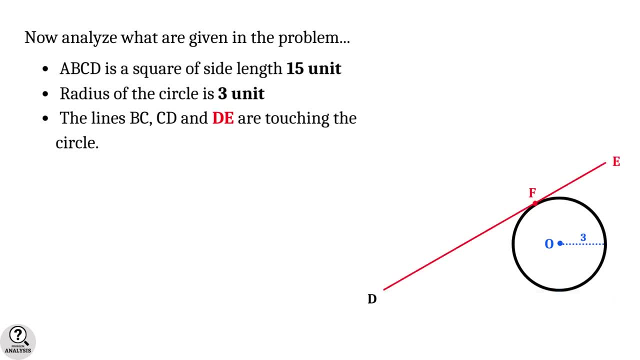 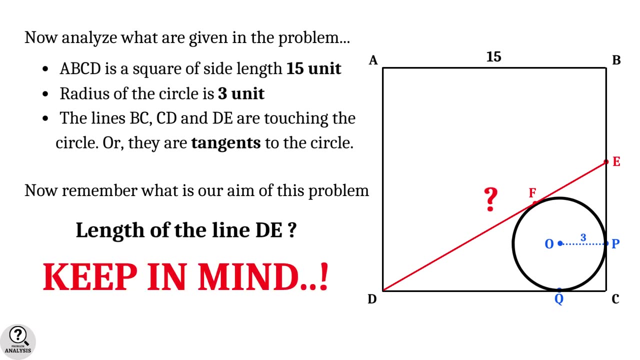 the circle at the points P, Q and F respectively. In other way, these lines are tandoms of the circle at those points. Now, what exactly is our aim of this problem? It is nothing but to find the length of the red line DE. This is the structure of our problem, So always keep in mind. 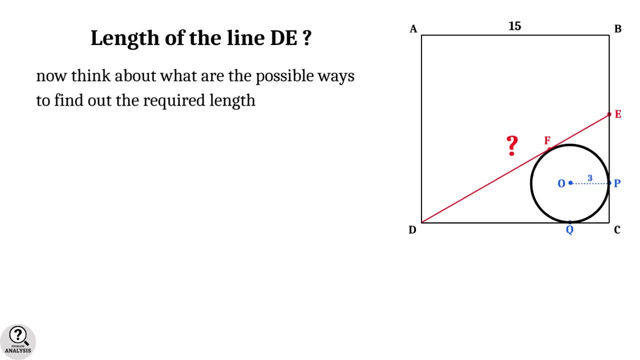 Now just think: how can we find that length? By a simple observation we can see that the triangle CDE is 3V. So okay, We have Que Crit, so we can find c critical. we have XO, then we have YC S or 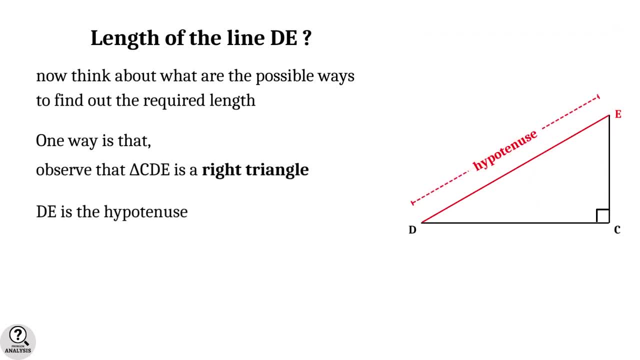 a right triangle and the red line, DE, is its hypotenuse. Also, we know that the base length is 15 units because it's the side of the square And that's it. So if we are able to find the length of CE, then by applying Pythagoras theorem, our answer is there. Let's proceed. 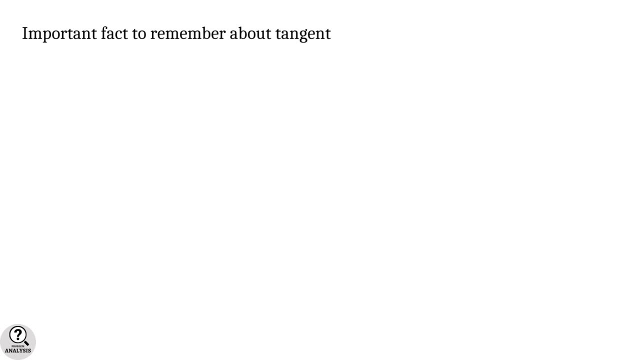 in that way, Before going to do the calculations, we have to remember an important property of tangent lines. Consider a circle and an arbitrary point L outside the circle. From this point we can draw exactly two tangents to the circle, And the fact is that they are. 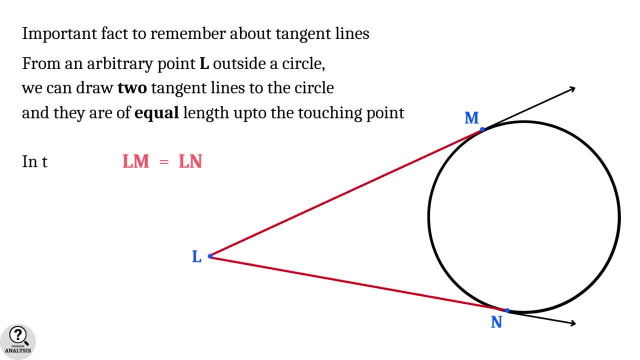 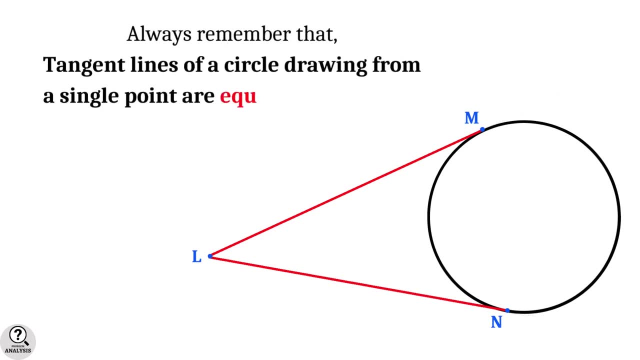 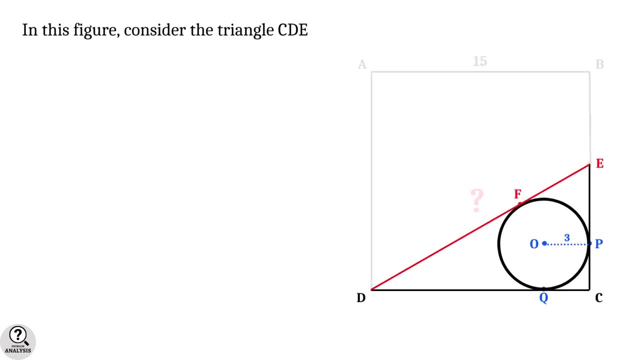 equal in length up to the touching points, That is, in this diagram, the lines LM equal to LN. To sum up, the tangent lines of a circle drawing from a single point are equal in length up to their touching points. Now, coming back to the problem, let's consider the right triangle. 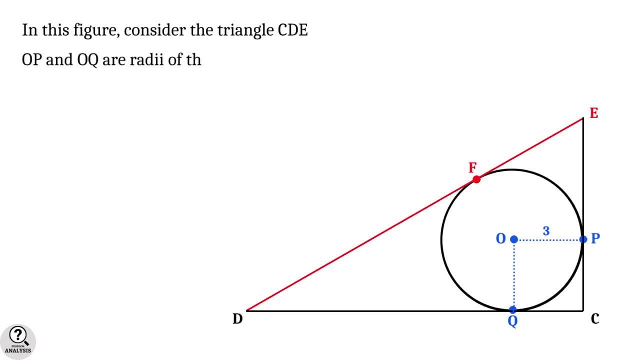 CDE. Clearly, the lines OP and OQ are radii of the circle, Which implies they are equal to 3 units. So it is clear from the figure that PC and QC are also equal to 3 units. Or in another way we can see that these lines are in fact two tangents. 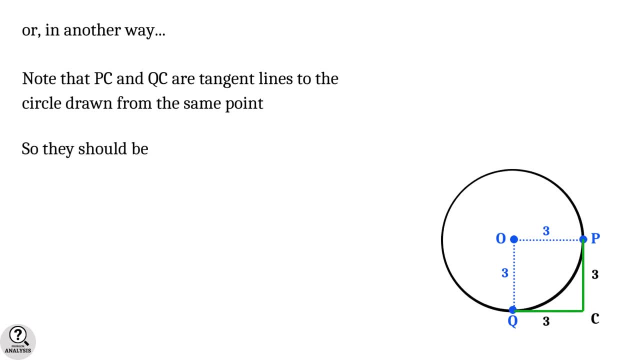 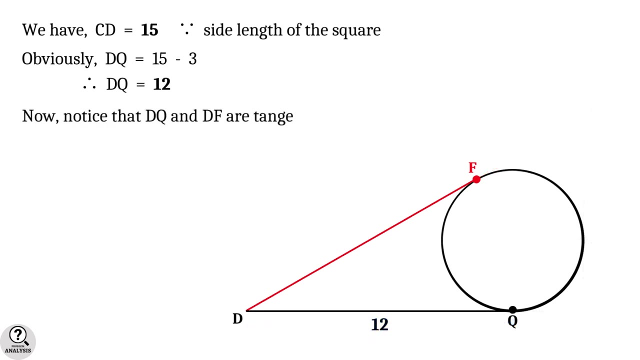 drawn from a single point, Therefore, by the property of tangents, they should be equal. Now we already have the side CD equal to 15 units. That implies DQ equal to 15 minus 3 equal to 12 units. Now observe the lines DQ and R3.. We can see that the lines DQ and R3 are equal to 3 units. Now we can see that the lines DQ and R3 are equal to 3 units. We can see that the lines DQ and R3 are equal to 3 units. Now observe the lines DQ and R3 are: 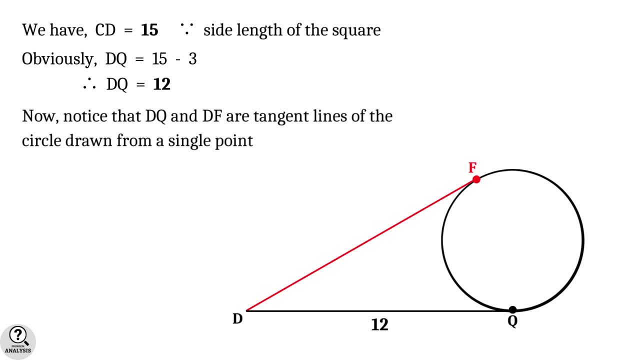 and df. They are in fact a pair of tangent lines of the circle drawn from a single point, which means they are equal in length and therefore df equal to 12.. The same argument can be applied to the lines ep and ef, because they are also a pair of. 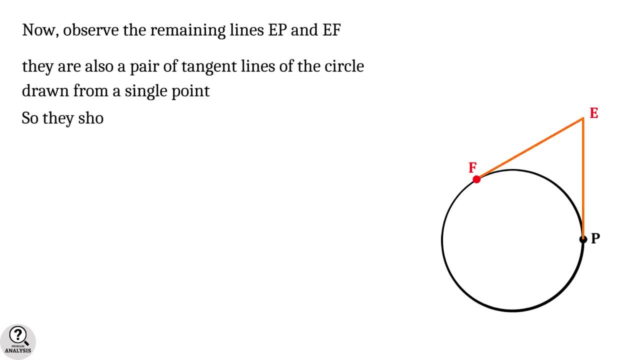 tangent lines to the circle from a single point, so they should be equal in length. Let's take this length as x units. That is, ef equal to ep equal to x units. Now we have all the sides of the right triangle: The side cd equal to 15, the side ce equal. 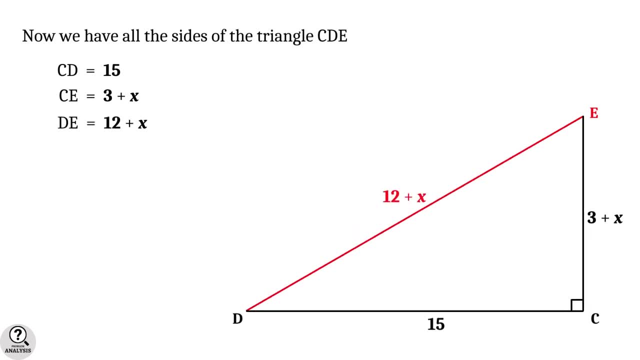 to 3 plus x and the side de equal to 12 plus x. By applying pythagore's theorem we get cd square plus ce square equal to de square. That means 15 square plus 3 plus x whole square equal to 12 plus x whole square. 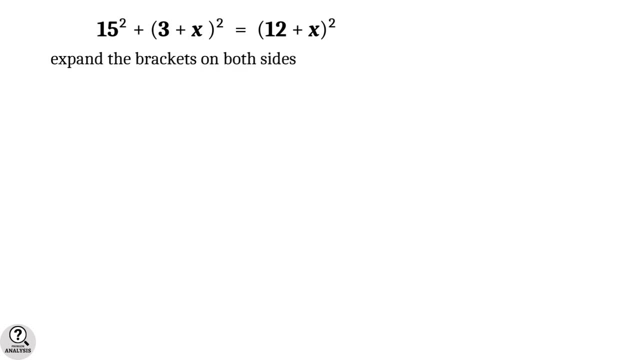 Open the brackets and expand the equation. That gives 255 plus 9 plus 6x plus x square equal to 144 plus 24x plus x square. The term x square cancels. What remaining here is 234 plus 6x equal to 144 plus 24x. 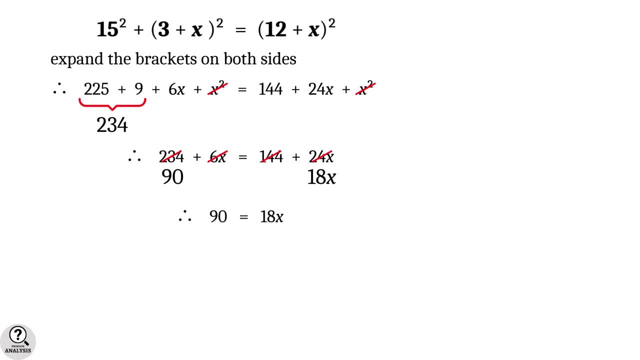 On simplification, we get 18x equal to 90. That is x equal to 5 units. Now we have to calculate the sum of all the sides of the right triangle. This is the result. What does it mean? We have the red line: de equal to 12 plus x. That implies de equal to 12 plus 5, which is: